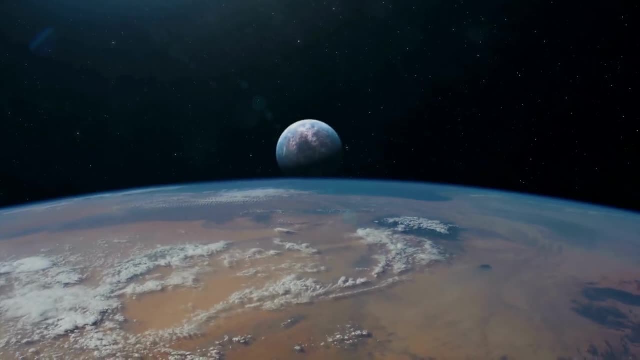 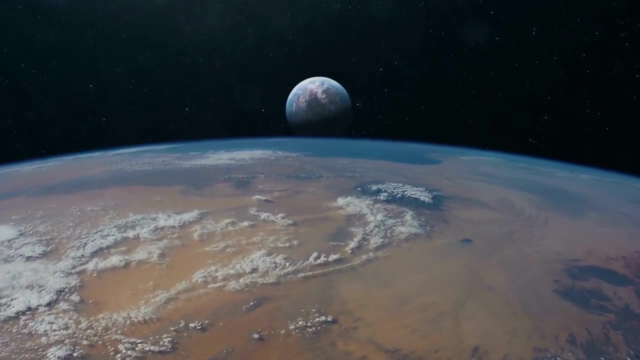 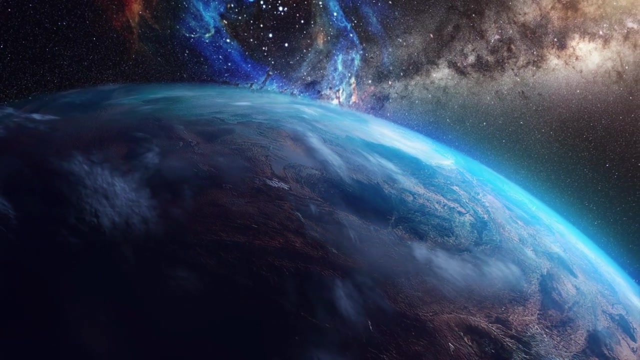 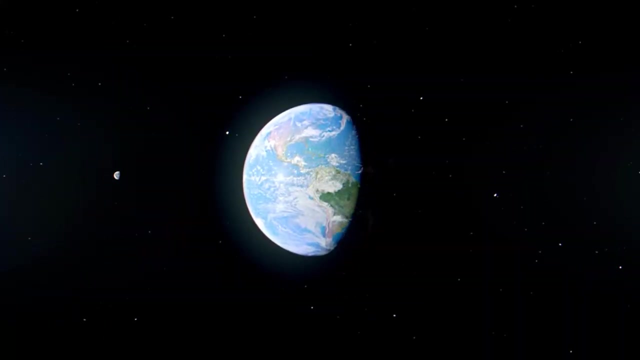 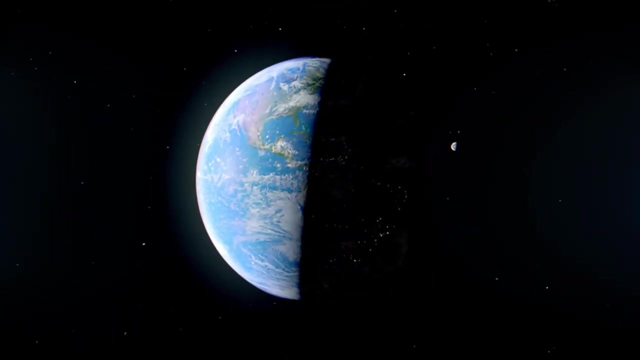 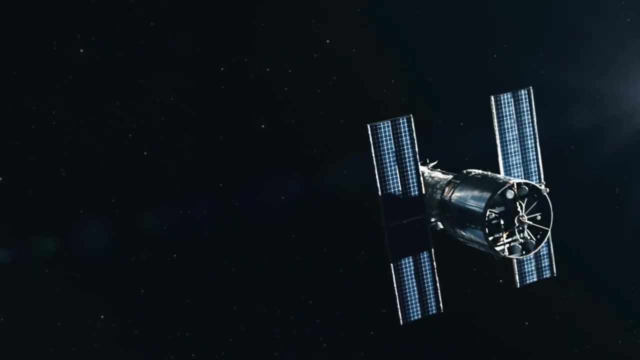 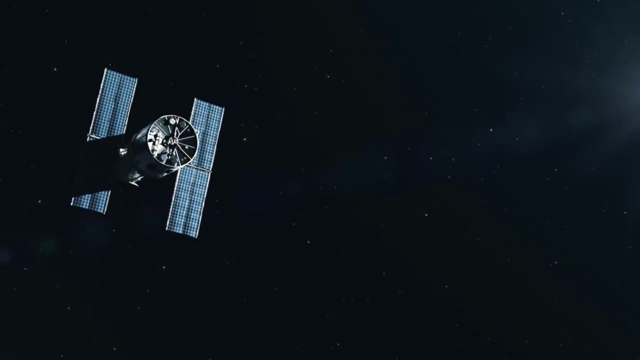 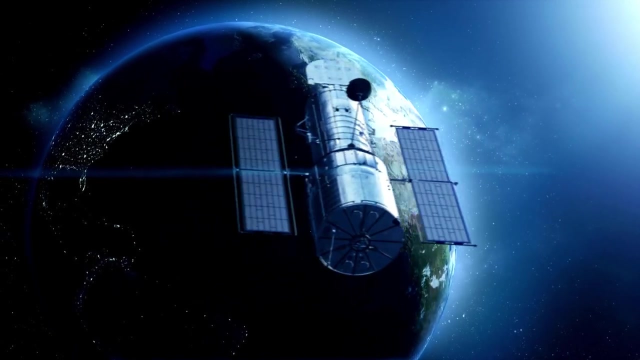 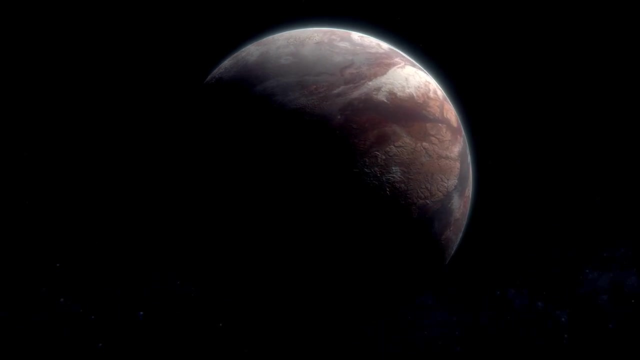 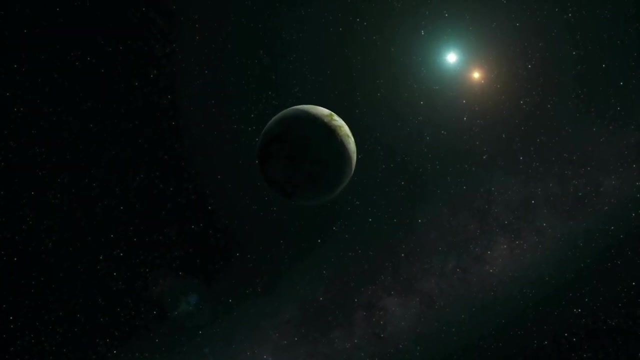 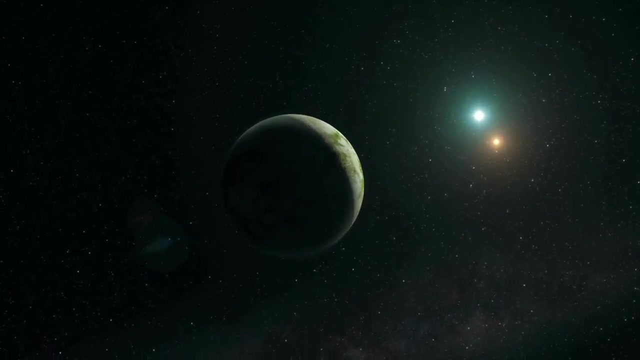 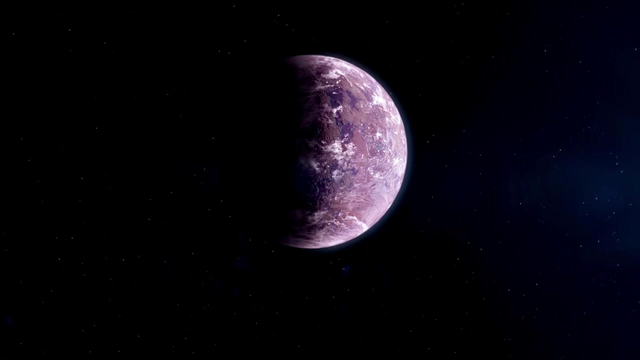 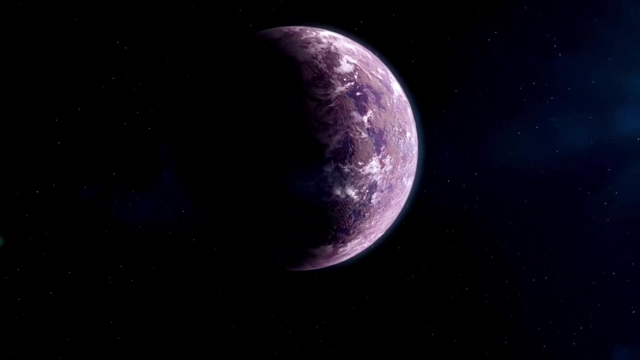 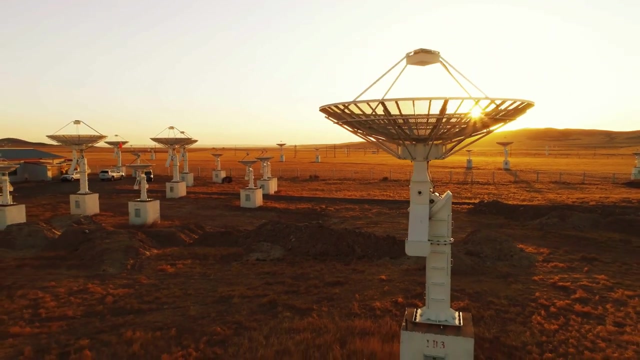 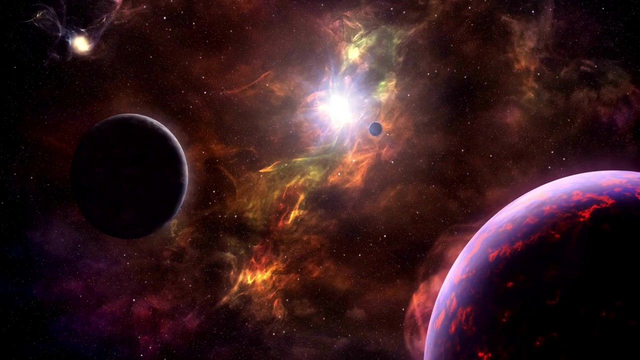 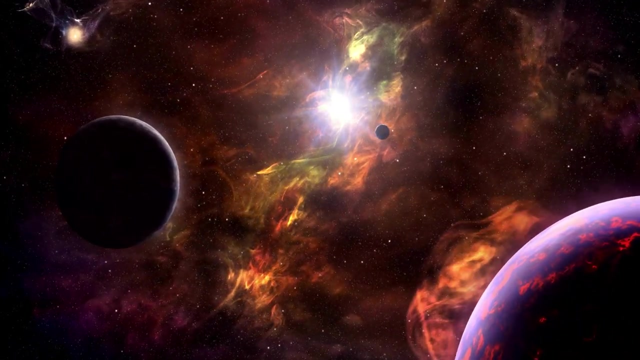 Thank you for watching. Thank you for watching. Thank you for watching. Telescopes with adaptive optics systems produce sharper images, allowing astronomers to distinguish between planet and starlight. Ground-based or space-based telescopes equipped with coronagraphs can block the star's light in the same way that you might shade your eyes from direct sunlight, making it easier to spot planets. 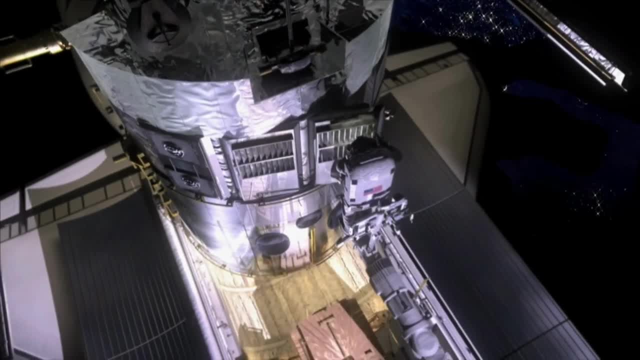 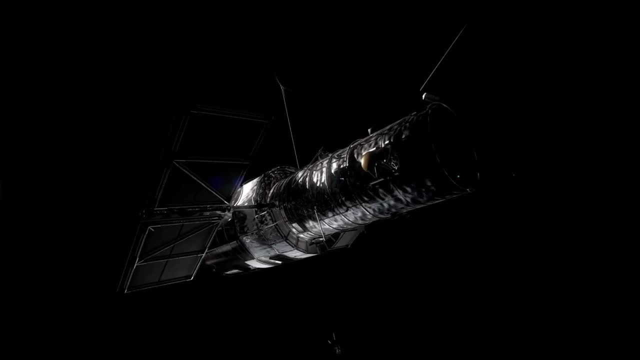 Missions to fly a star's shade in formation, with the telescope blocking starlight before it reaches the imaging system. Missions to fly a star's shade in formation, with the telescope blocking starlight before it reaches the imaging system. One of the most obvious benefits of direct imaging is that it produces fewer false positives. 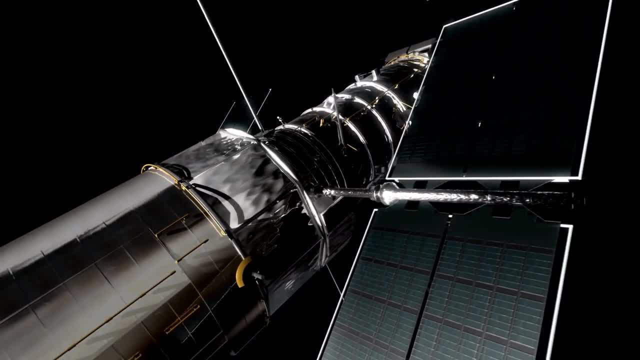 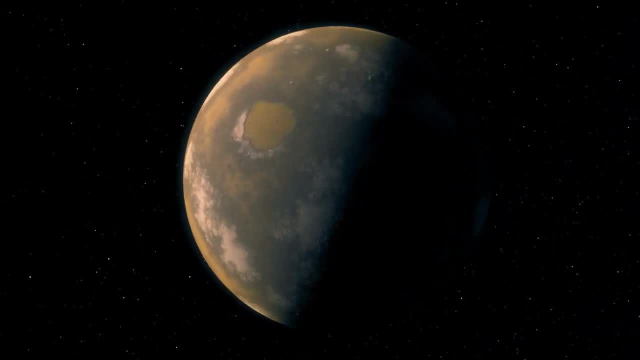 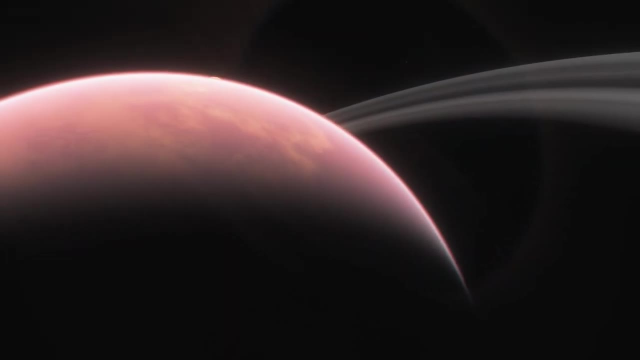 Scientists can learn a lot about the planet by using direct imaging. For example, in the case of Fomalhaut b, the planet's interaction with the protoplanetary disk and the fact that it is invisible in the infrared provided strong limits to its mass. 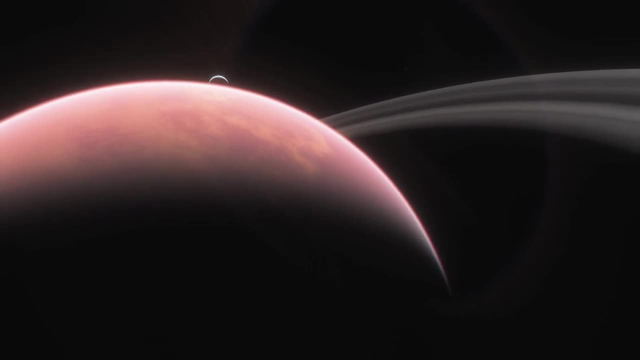 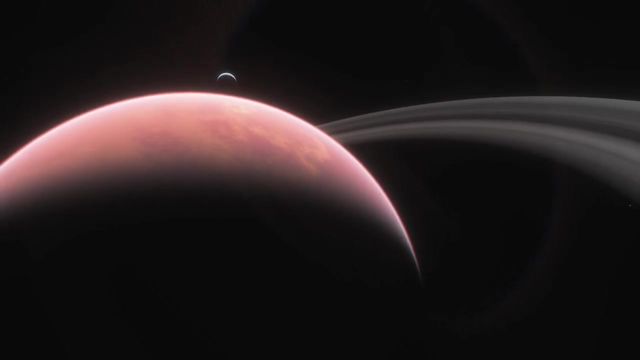 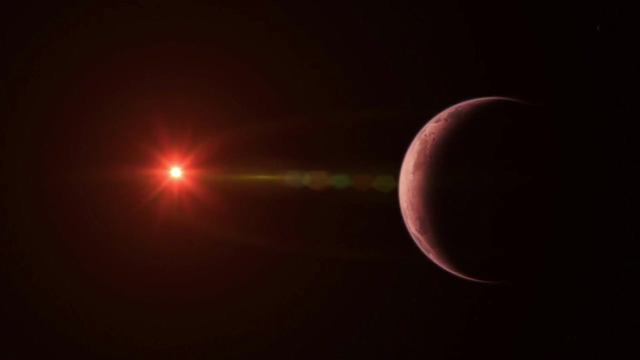 and its exceptional brilliance led scientists to hypothesize that it is surrounded by a massive ring system. In the case of HR 8799,, infrared radiation from the objects, combined with planetary formation models, yields a rough estimate of the planet's mass. Direct imaging works best for planets with large orbits and a high mass, such as gas giants.